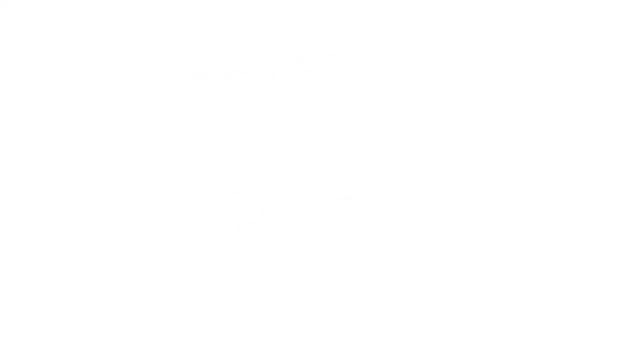 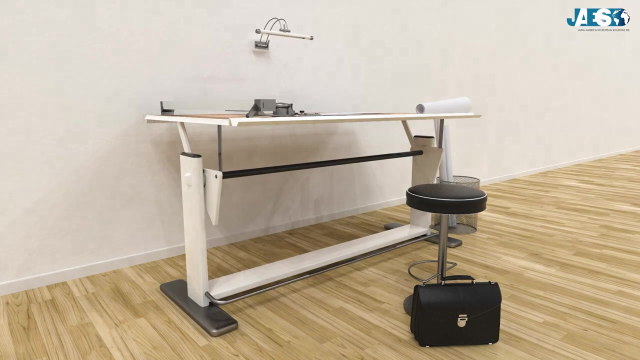 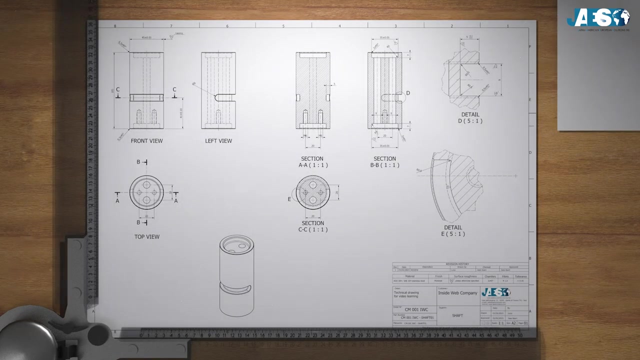 In engineering, when an object is designed, a technical drawing is used to represent it graphically on a screen or sheet so that engineers, workers and users can communicate with each other and understand what it looks like. In this video, we will look at the basics. 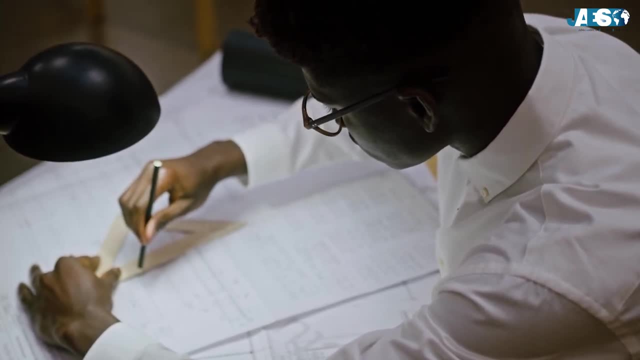 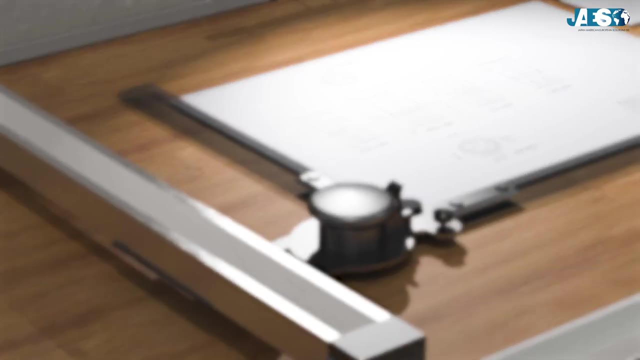 of learning how to read a technical drawing so that, in just a few minutes, you can correctly interpret the various elements of it. There are various regulations that define guidelines for producing technical drawings, such as the International ISO System, But in this video, 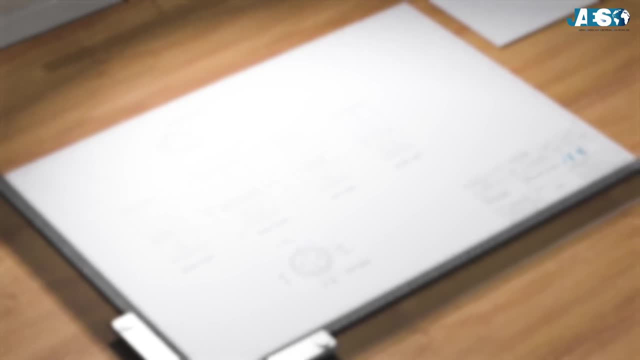 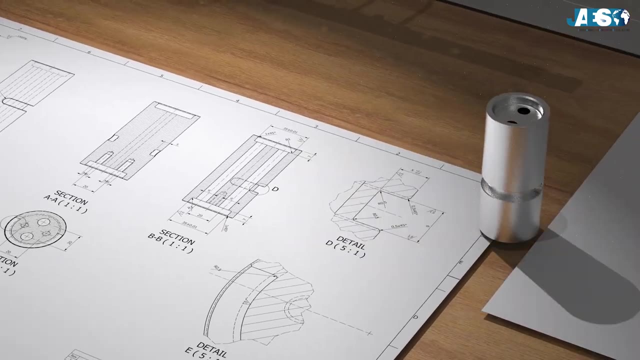 we will only look at the basic principles that are generally common to each standard. Let's take a very simple object. This shaft has many features. Let's look at its engineering drawing In order to represent the object on a sheet of paper, some of its projections are: 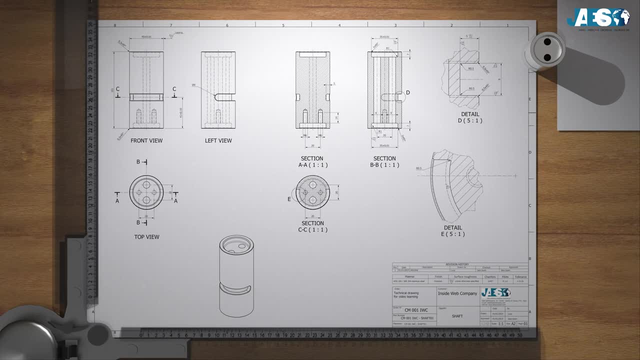 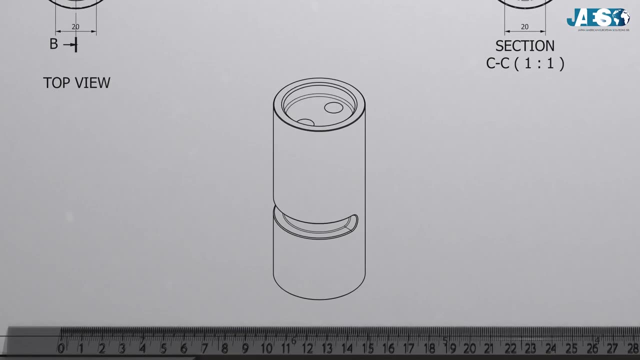 required. In other words, the shaft has many features. Let's look at its engineering drawing Graphic representations that describe the object As it can be seen. there is its three-dimensional representation, an aid not always present for immediately understanding the shape of the object. The projection is in isometric axonometry, meaning that the XYZ axes 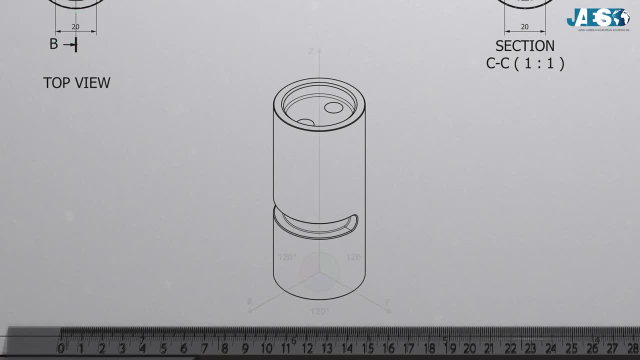 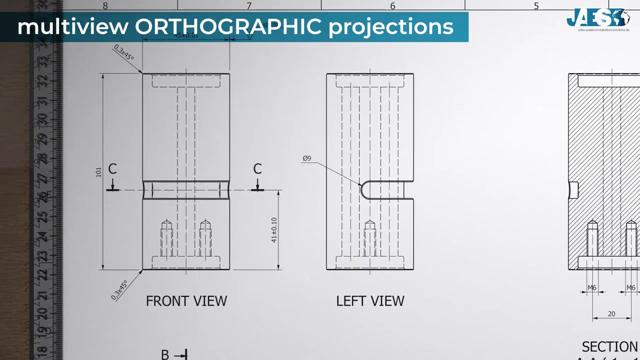 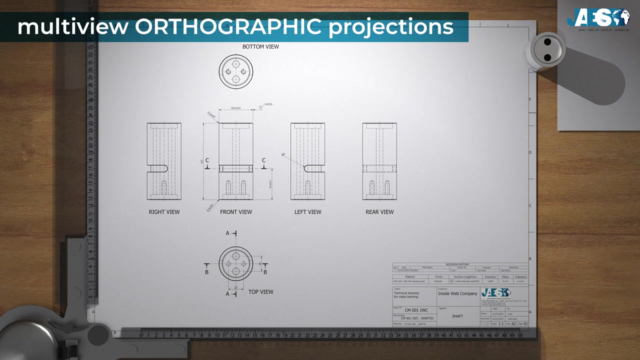 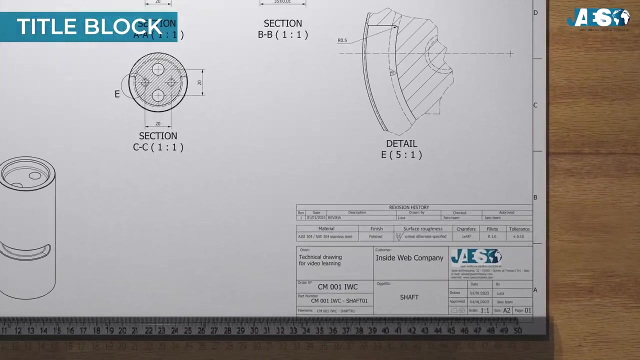 form three equal angles of 120 degree. Then we have the multi-view orthographic projections. To understand the shape of this object, we need three of them. In essence, there are up to six two-dimensional images representing perpendicular views of the object. But the first thing to do to understand orthogonal projections is to read the title. 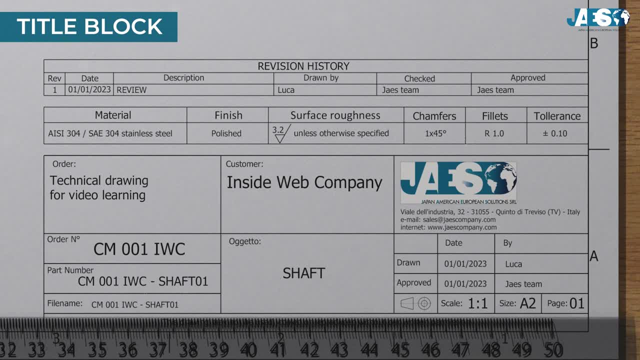 block a table, usually in the lower right corner, in which all the primary information is enclosed. It usually includes the company logo and the designer's name to know who to contact, a title code or drawing number and anything else needed to identify the object and track it down. usually, 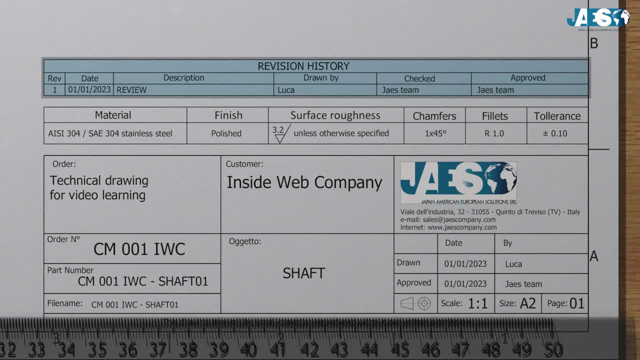 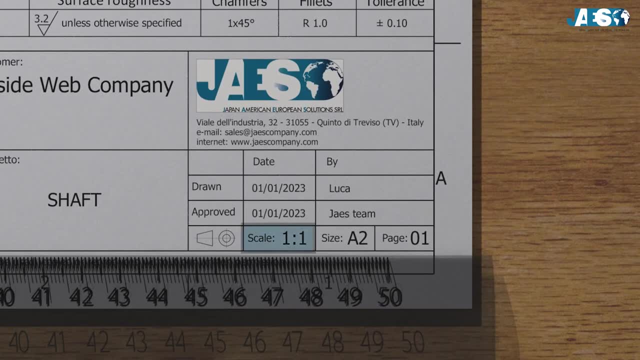 in a separate cartouche the revision number and date to tell if it is the latest version of the drawing and when it was made. Then there are the scale of the drawing and the paper size it needs to be printed on to get the correct scale. These two pieces of information are related. 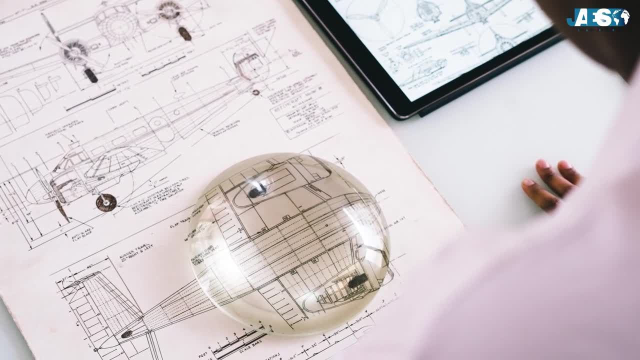 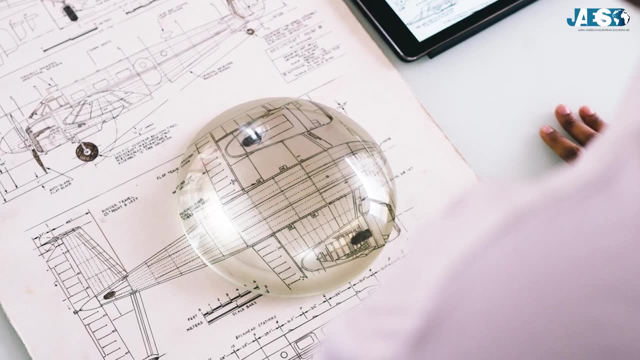 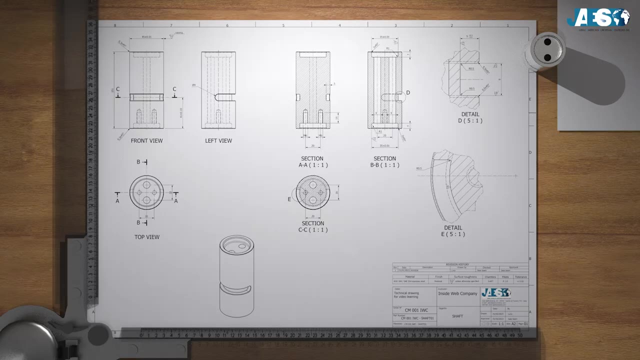 The drawing of an object most times doesn't have actual dimensions, but they are scaled to fit into dimensions of a sheet. if the sheet is printed in the indicated format, then the scale will be correct. in this case the scale is one to one. it means that actually the drawing is in full scale. 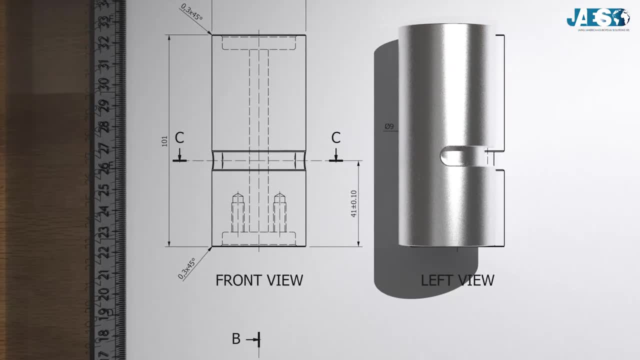 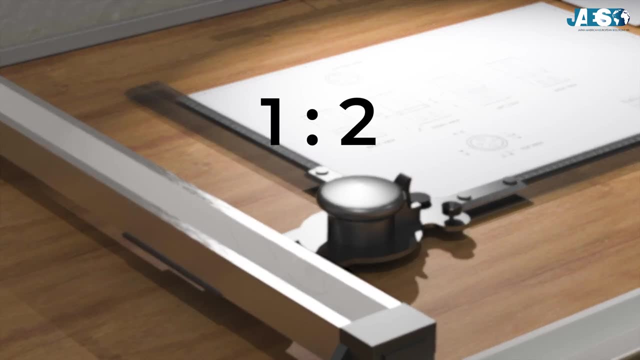 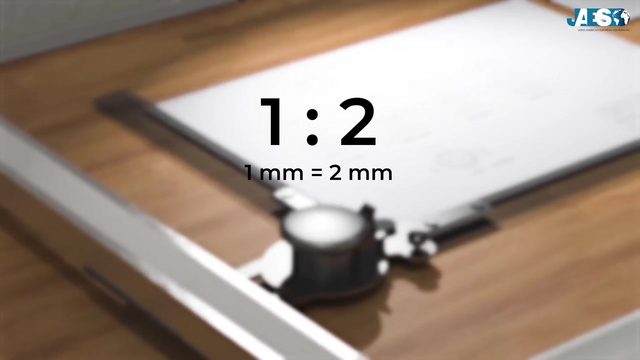 and has the same dimensions as the real object. so if we take measurements directly from the sheet by means of a ruler, these will be effective, while if it is written, for example, scale one to two, it means that the object is drawn, reduced by half of the real size. in practice, the dimensions we 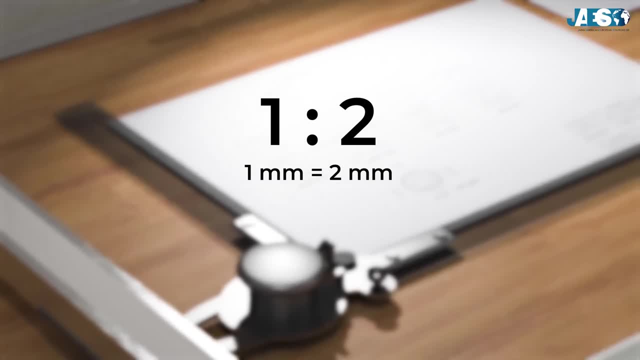 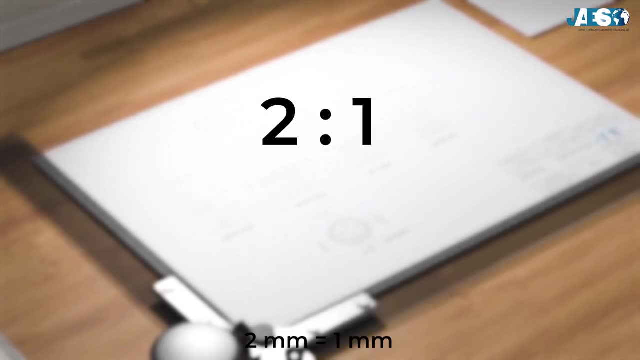 measure will have to be multiplied by two to understand how big it really is. on the other hand, if it is written two to one, we are dealing with an enlargement. the object would be drawn twice as large as it really is. so we have to divide the measured measurements by two. 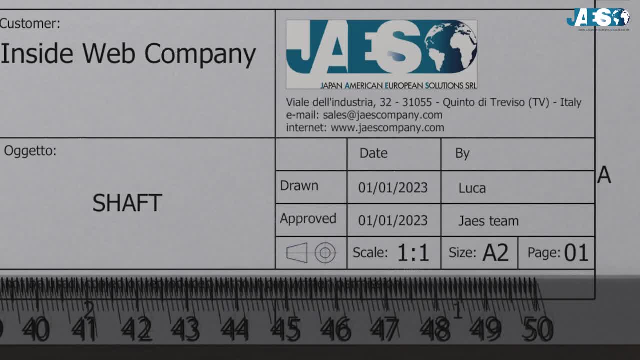 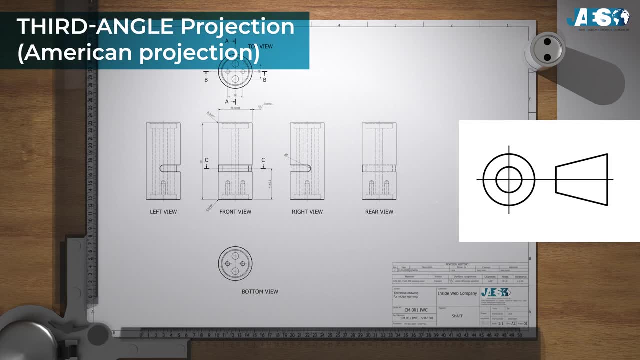 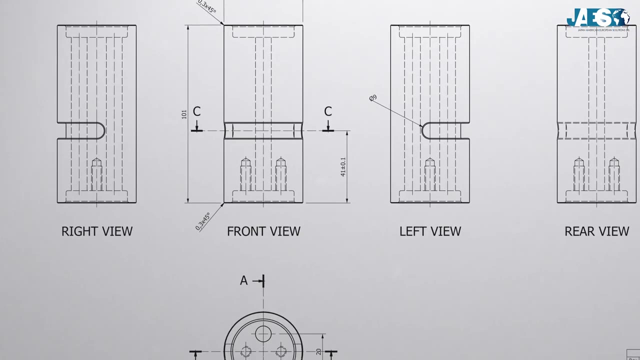 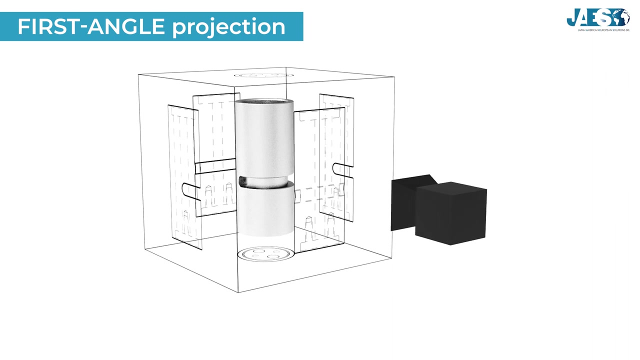 another fundamental thing is the symbol to define whether the orthogonal projection used is of the first angle or the second angle of the sheet. the orthogonal projections are not randomly arranged. they are aligned with each other by one of these two standards. with the first angle projection, the object lies between the observer and 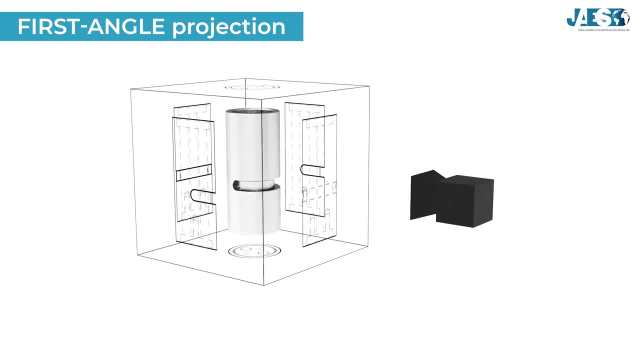 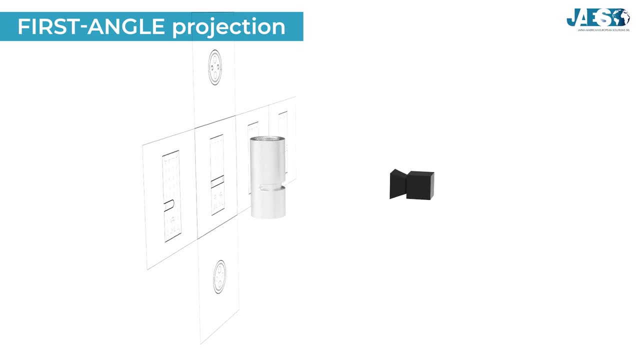 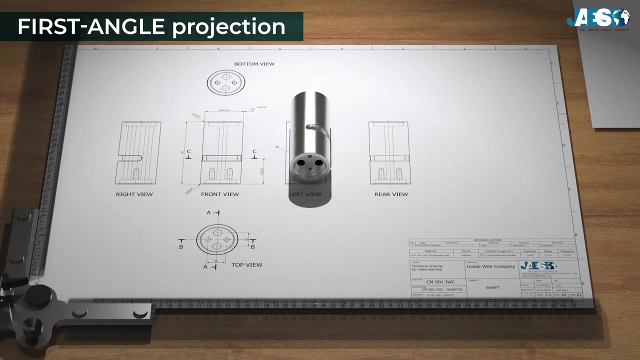 the projection planes by imagining a cube surrounding the object. each view is projected onto the inner walls of the cube, which is then unfolded into a square shape order to create all views. For simplicity, it is like laying the object on the paper and rolling it to arrange the 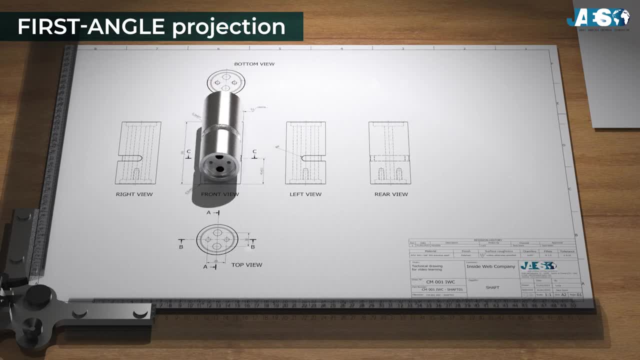 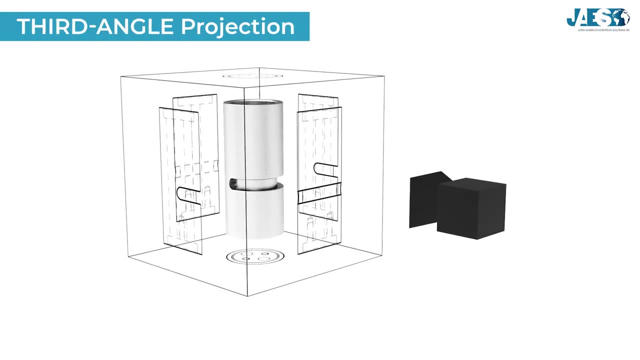 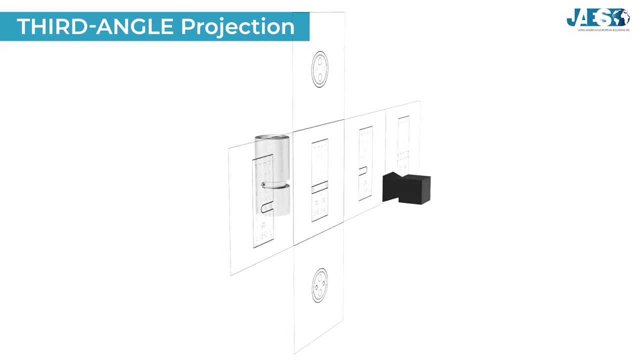 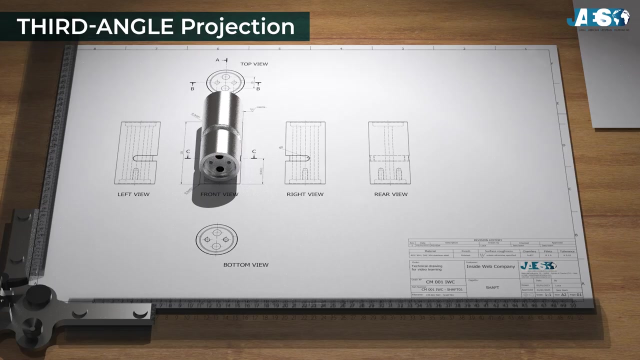 various views. In contrast with the third angle projection, it is the projection planes that are between the observer and the object Imagining the cube surrounding the object. each view is projected onto the outer walls of the cube to then be unfolded, For simplicity, starting from the front view. we have its right view: top view, above, bottom. 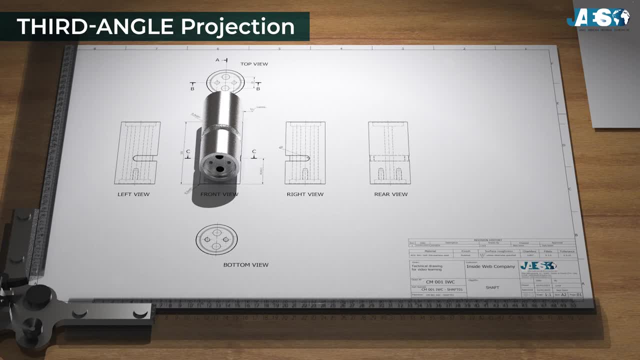 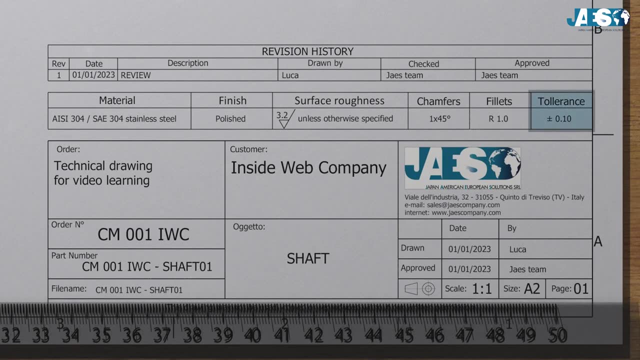 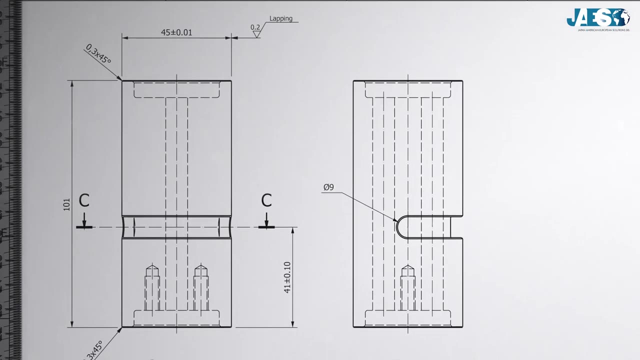 view below, etc. The exact opposite of the first angle projection, General tolerance, is also present In orthogonal projections. there are dimensions, numerical values that are the actual dimensions of the object and which are expressed in millimeters in mechanical drawings At the time of production. where one cannot, 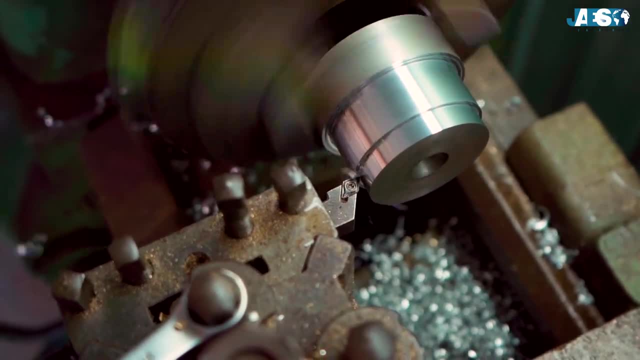 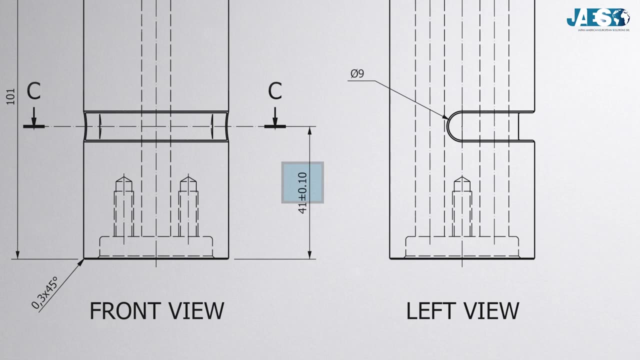 expect absolute perfection. this data allows one to understand how precise the manufacturing must be. In this case, where it says ±0.10,, it means that the tolerance is two-tenths of a millimeter. so in this 41-millimeter dimension it's accepted a manufacturing error that can be. 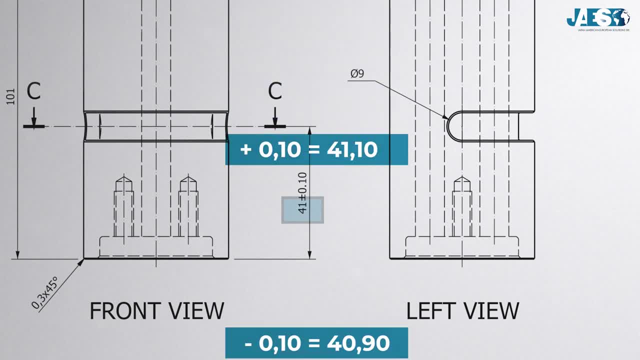 ±¹⁰, that is, 41.1,, or ±¹⁰, that is 40.9.. A tolerance can also be specific. The tolerance may be a total of 0.1.. The tolerance can also be specific to a given dimension. 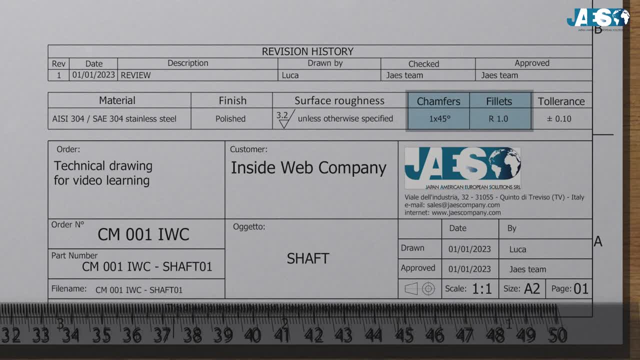 Similar to the above. there are undimensioned fillets and chamfers. These general figures must be taken into account, unless a fillet or chamfered edge is specified in the dimension. Lastly, there may be additional lines which specify finish, surface roughness or other. 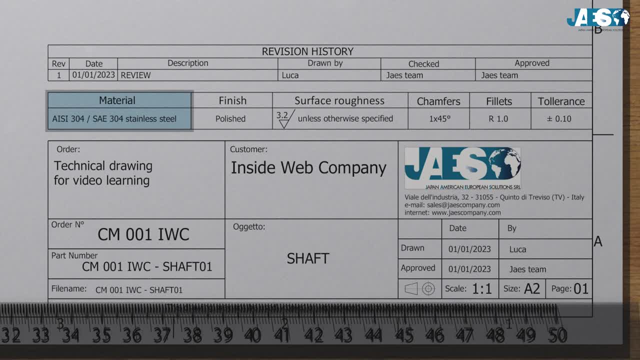 features of the part that cannot be drawn, such as the material which, in this case, as the acronyms of the AIC and SAE designation system, is not included, say is common 304 stainless steel. now let's move on to the actual drawing as: 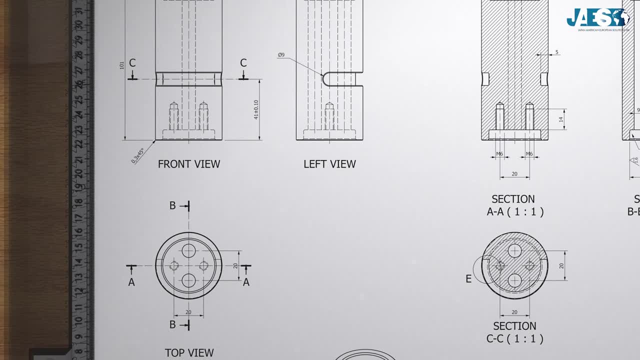 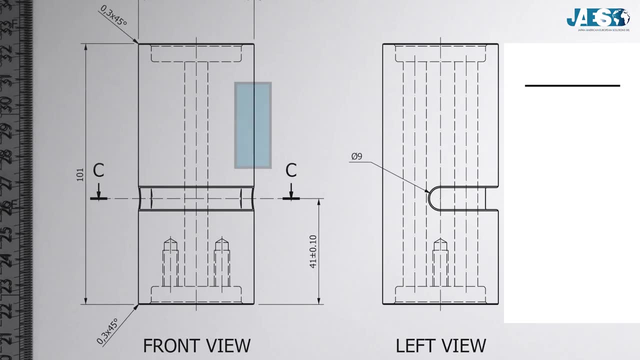 we can see, it is made up of different lines of different thickness, continuous or dashed. each one has a meaning. the thick line defines all the contours and edges that can be seen in that view, while the dashed line shows those that cannot be seen in that particular view. a dashed dot line, on the other hand. 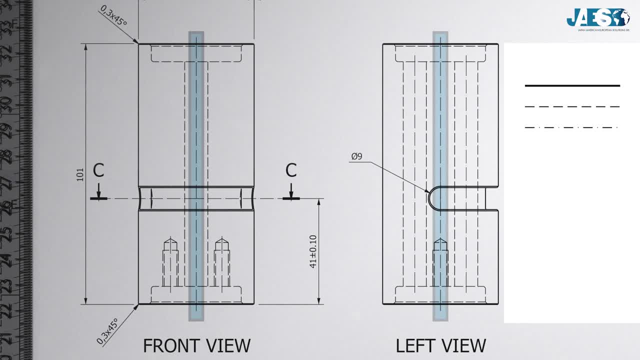 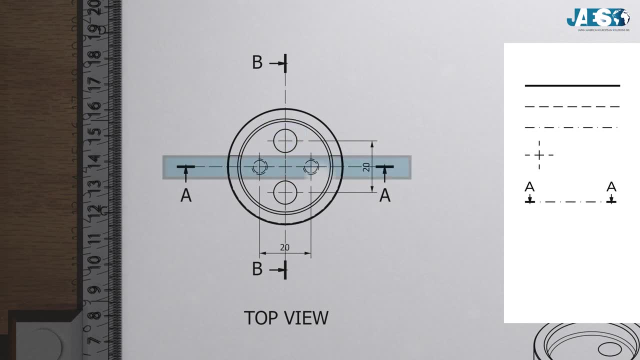 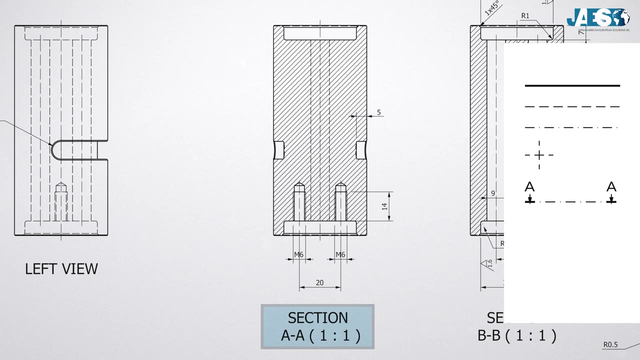 indicates symmetry if the object on either side of the line is substantially mirrored. they are also used for holes. a dashed dot line may also indicate a section if there are arrows indicating the direction of the view and letters that are shown in the actual section. drawing a section is an internal view of 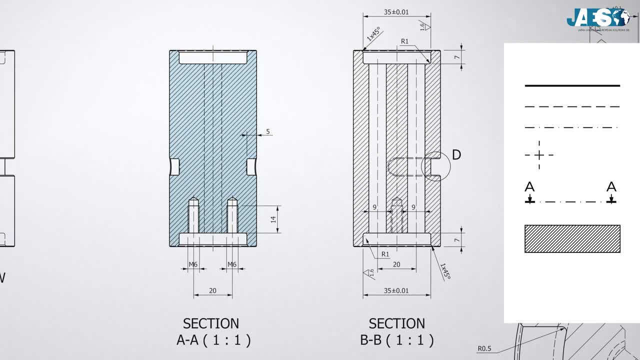 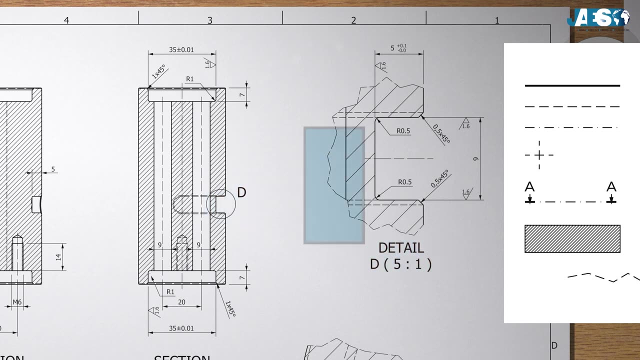 the object. if we're looking at it, there are crossed out fields with 45-degree lines representing the internal surface of the object, as if they were the cut surface of the solid, while a detail is an enlargement of a certain area, always named by letters, where usually irregular lines interrupt. 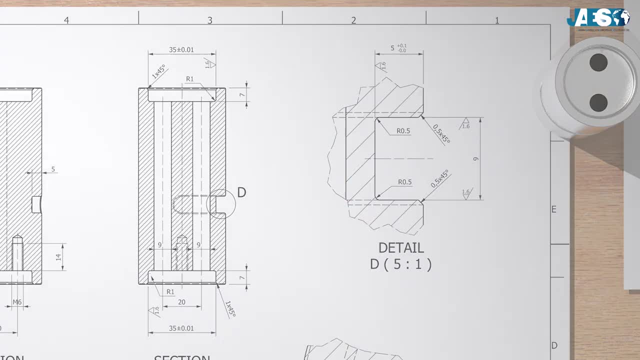 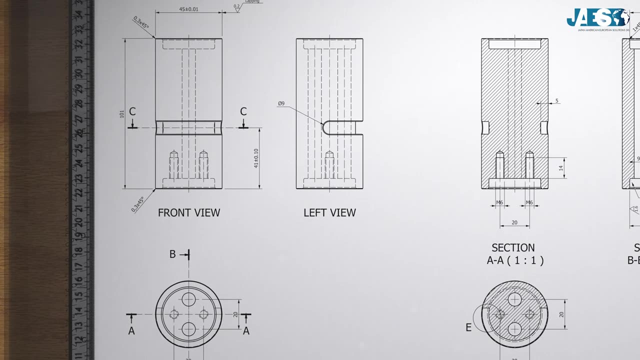 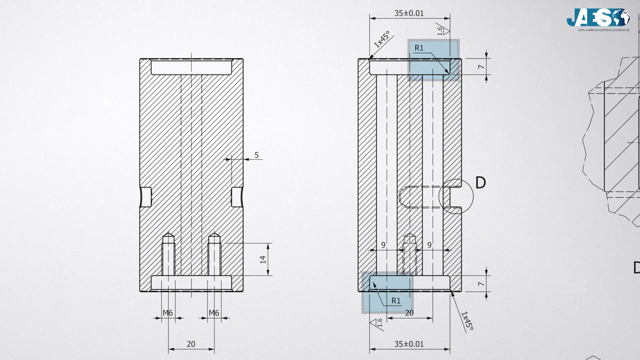 the drawing, leaving only the necessary parts. dimensionings, on the other hand, are represented through thin continuous lines which, placed side-by-side with numerical values, can indicate lengths of the various parts of the object: fillets, if the letter R is present. diameters, if the symbol Phi is present. 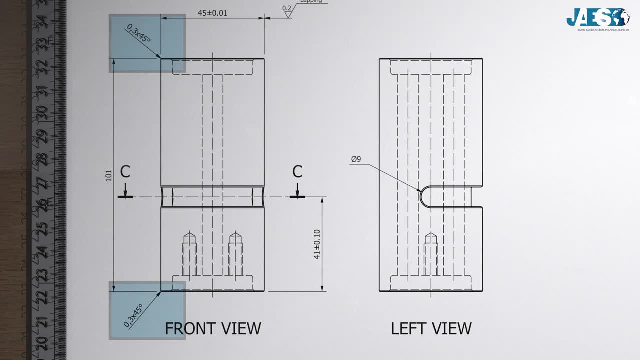 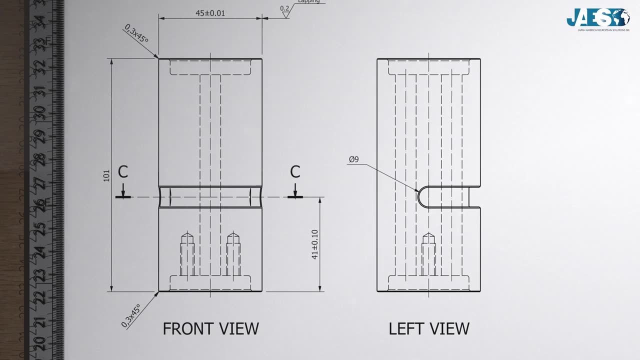 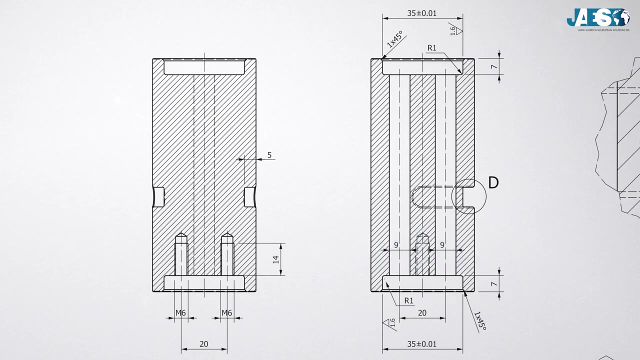 chamfers by specifying the height and degree of inclination. they should always be arranged externally in relation to the projection and can be attached to visible lines and axes of symmetry. therefore they are placed internally only if necessary and hidden lines are not dimensioned for these reasons. there 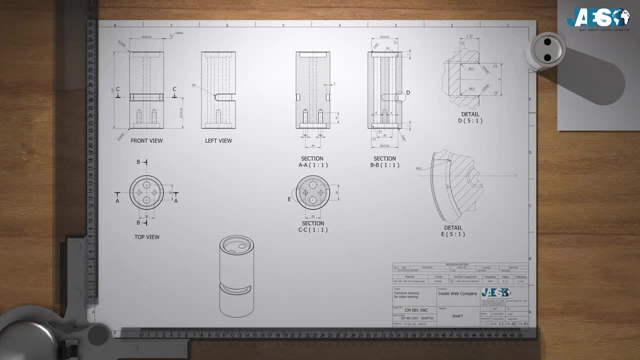 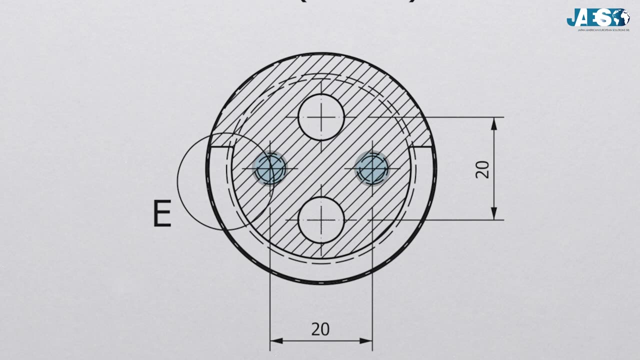 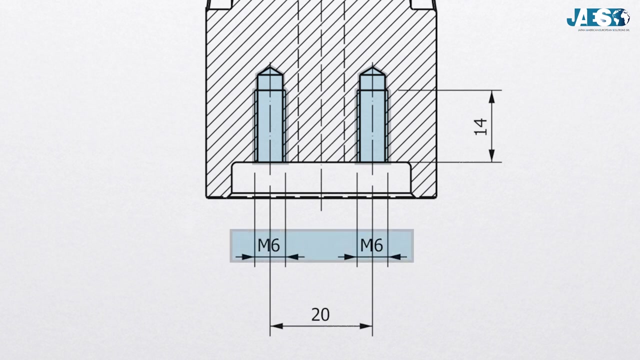 exist other views and sections. threaded holes, on the other hand, are represented as two concentric circles representing the root and crest of the thread. usually, threaded holes are defined according to the ISO standard, which consists of an abbreviation, in this case m6, which specifies the diameter of the hole to be made and the 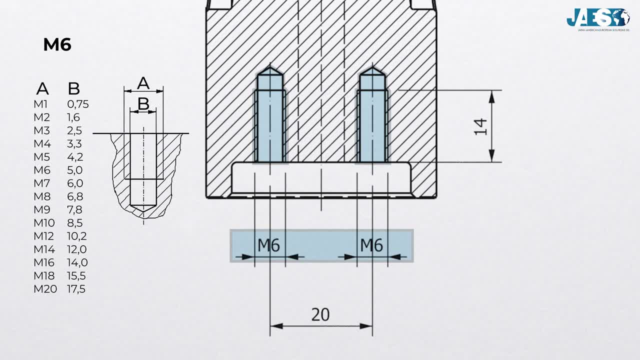 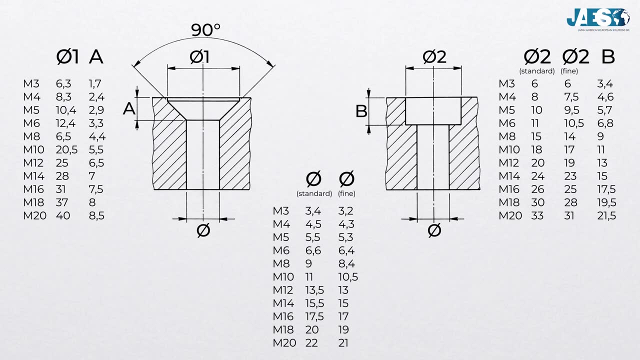 diameter of the thread to be made inside it. after an X, the fine thread may be reported. if it is not present, it is implied that you are using the course thread, and after another X, the length of the threaded hole is reported. often the hole has a countersink or a counter bore that serves to accommodate the head of the 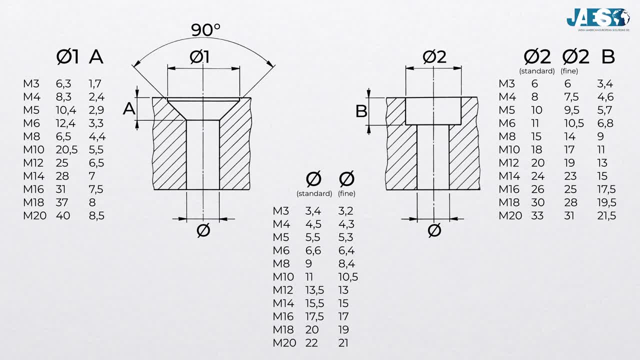 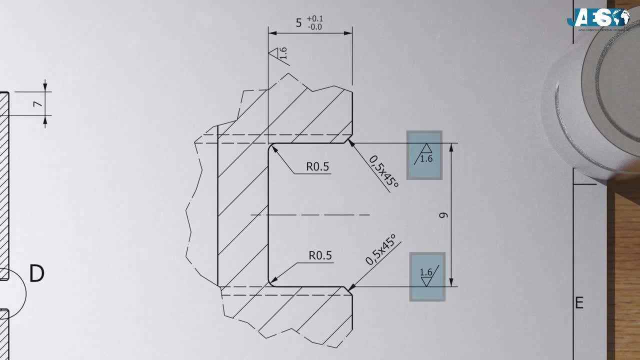 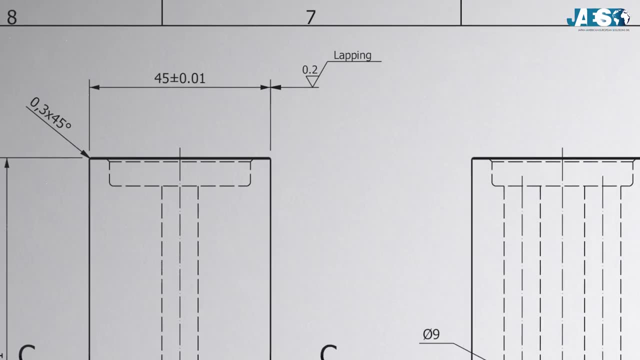 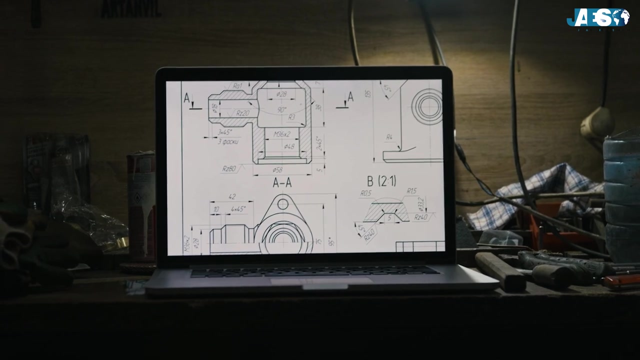 screw, which is specified with dimensionings and is standard according to the type of screw. along with the dimensions, one can also indicate the surface roughness index of that particular face, which may deviate from the general roughness index. finally, there may be notes for machining processes or warnings. now that you have understood the basic principles of 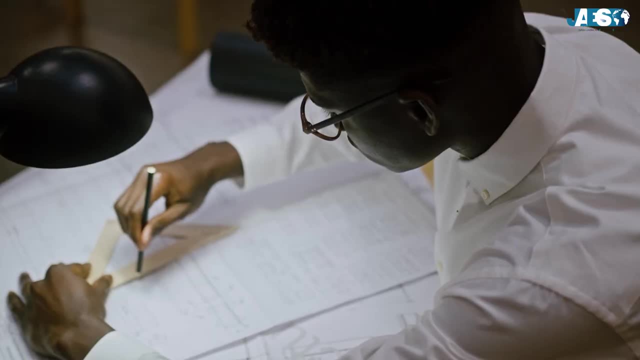 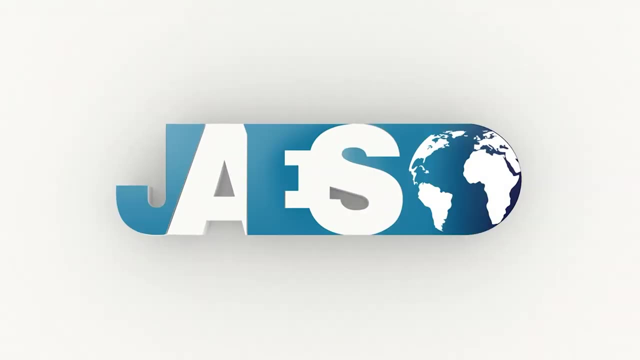 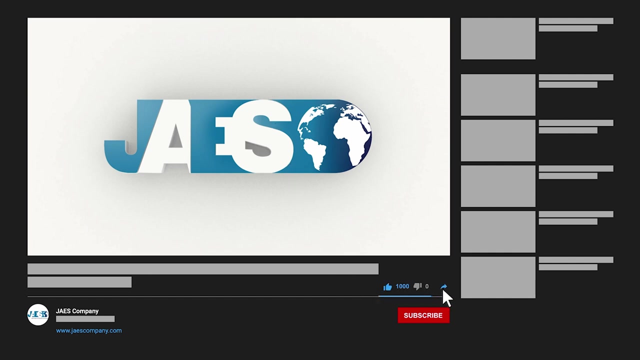 technical drawing. you can use it to create an object or design a project yourself. if you found this video useful, let us know by leaving a like and a comment. you can also share it, and don't forget to subscribe to our channel. we recommend you visit our website, JawsCompanycom, to know about our upcoming projects.